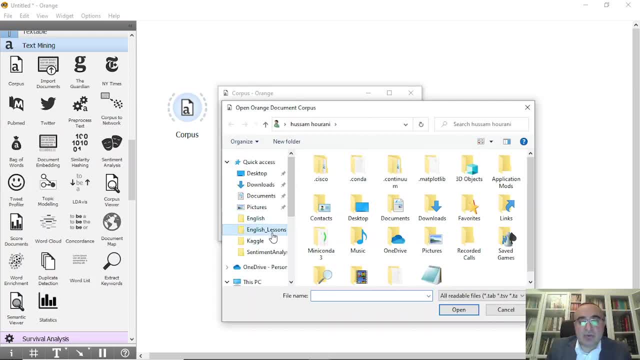 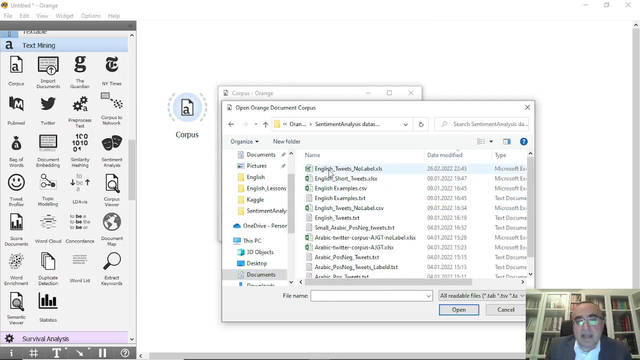 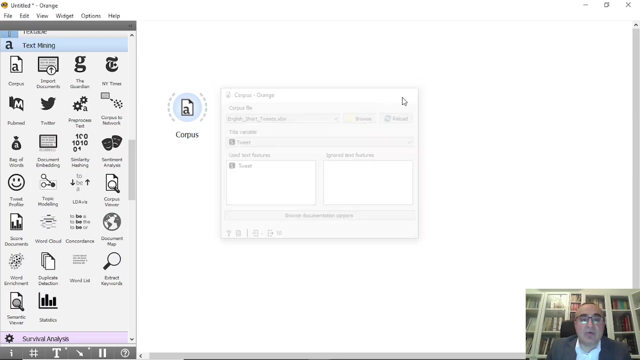 from corpus. what I'm gonna do? I'm gonna browse to a certain folder and I'm gonna select from sentiment analysis. I'm gonna use English tweet. English tweet this: this is the one English short tweets. English short tweets: we have tweet and we have also the tweet in the feature. now. 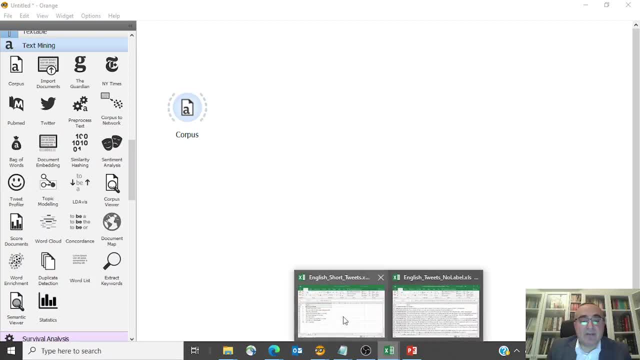 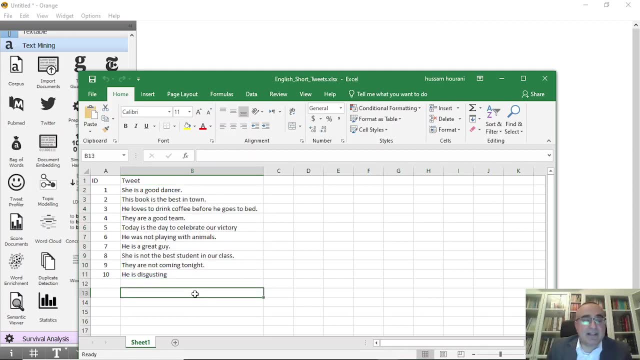 with this one. let me show you exactly which file I have have. I have chosen. this is the file we. so we have these tweets, very simple tweets, so I can explain what is sentiment is all about. so we have the id and the tweet, id number two and the tweet. the first tweet is: 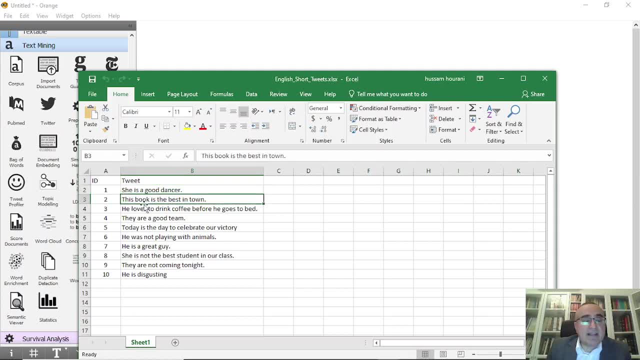 she is a good dancer. the second one is: this book is the best in town. the question: is: this statement positive or negative statement, or a neutral statement, neutral statement, or what is the combined between all these things? so the purpose of sentiment analysis is to analyze the statement, if it's positive statement, negative statement, neutral or the combine. so this is what. 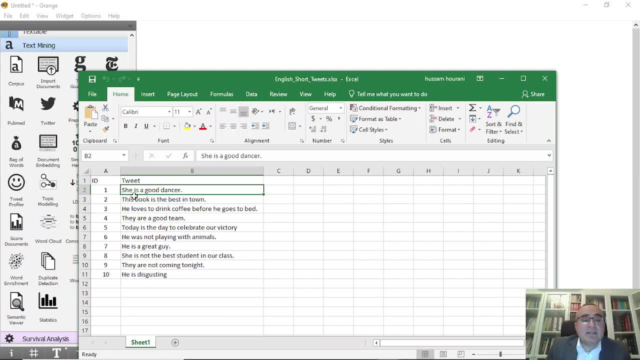 we're gonna do so, for from just reading this statement, you will judge that this statement is positive. she is a good dancer. now, if you read the last one, he is disgusting. this is a very negative statement. let's see how we can. we can identify all of this in orange data mining. so of choosing the 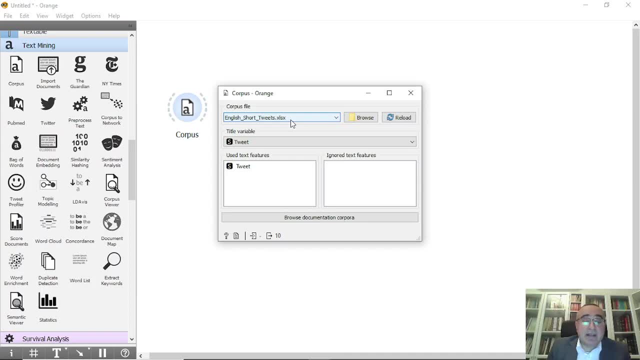 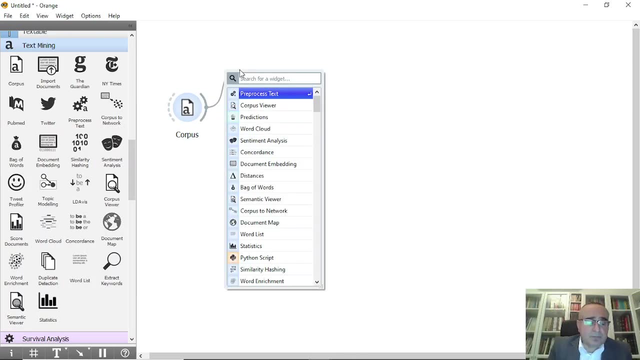 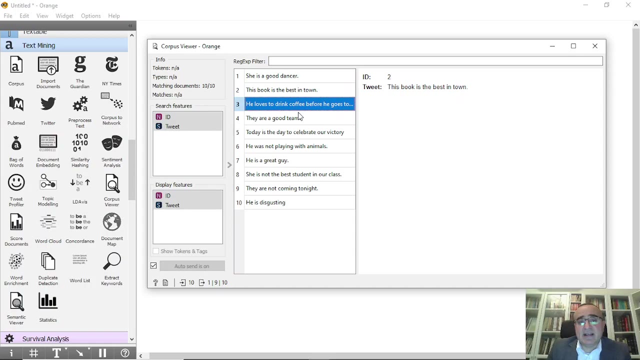 English short tweets with excel. I'm gonna keep this file in the github for you to download and try it. try it yourself. and from here you can do first one thing, which is corpus, corpus viewer. corpus viewer. okay, from corpus, you will see all these- uh, you know- statements, so you directly. 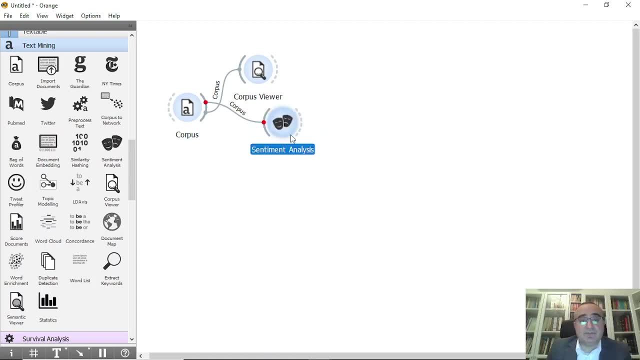 connect to sentiment, sentiment analysis, if you want, okay. and from sentiment you can choose which language you would like to do, which sentiment method you would like to do. maybe, maybe we can use the vace for now, but you can choose the multi-sentiment and use the language which. 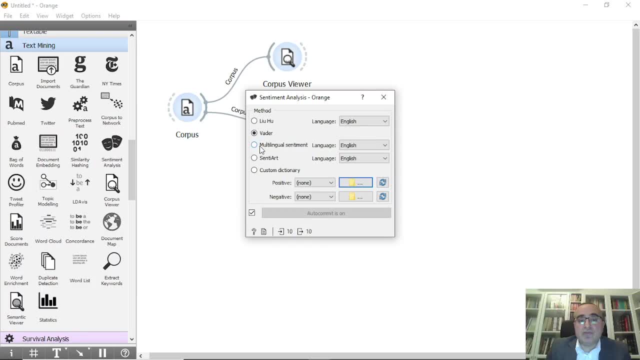 language you are dealing with. you can choose, for example, multi-sentiment analysis or vader- let's try this one- and the sentiment is done to view it. we can go, for example, into corpus viewer or data table, data table. see you from data table. this is what I want to do from data table. 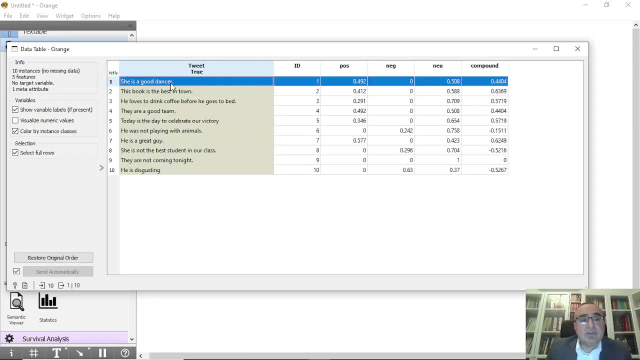 is the tweet: okay, he is a good dancer. and the positive is 0.49. okay, the negative is 0, so you can now understand that, or you can conclude that this is a positive statement. you can click on positive, negative and your and neutral, neutral, neutral or compound. so if you click and the positive, you will see. 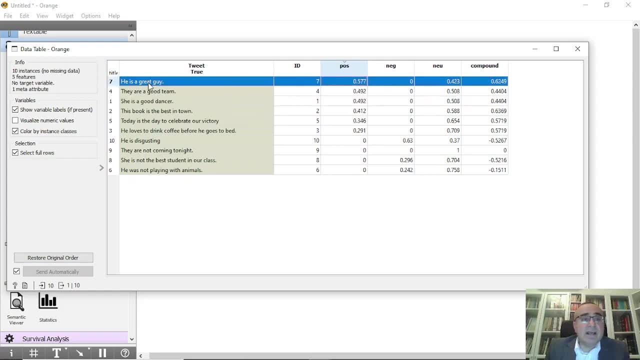 twice. the most positive word is: he is a great guy. this is a positive statement. of course, this is not a negative. so it's 0, the neutral it's 0.4 and the compound between all is 0.62. let us click on the negative. let's see the. 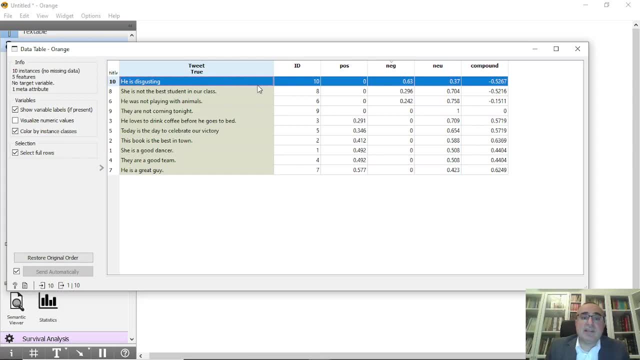 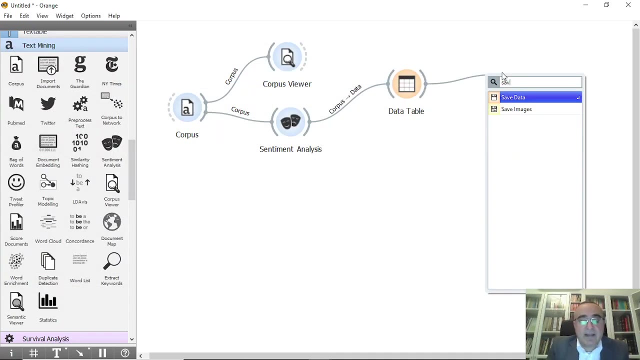 highest negative: 0.6. he is disgusting. so the negative is he is disgusting. so from this table we identified which statement is positive, negative, neutral or compound. we can identify and we can also set the whole thing now and to save file: okay, and we can put it in a report so we can click in the save save, as for example: 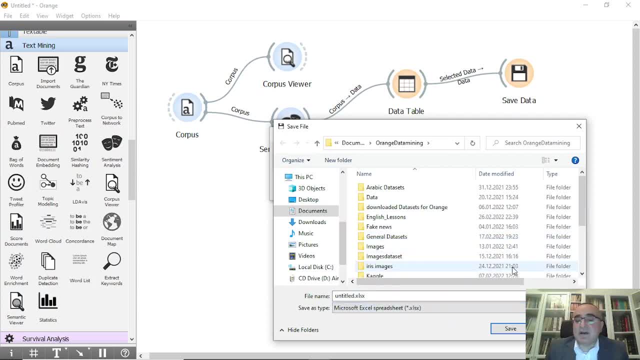 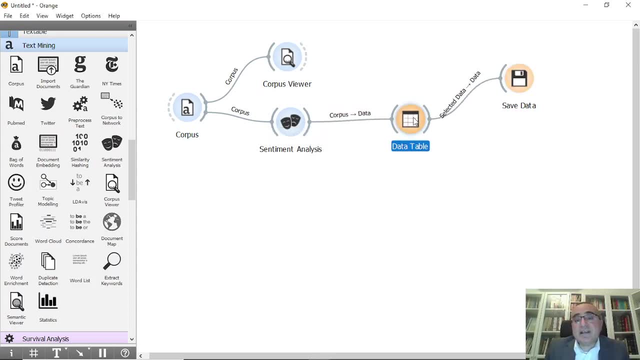 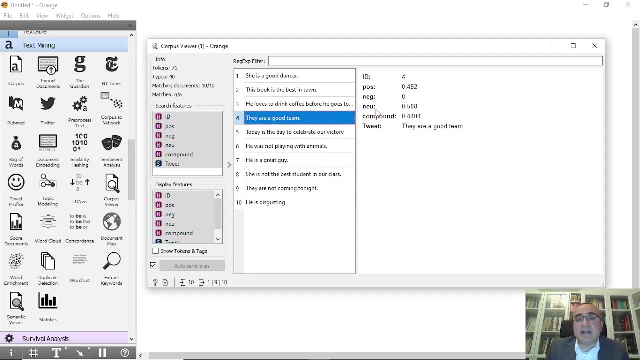 Excel. you can go to excel sheet or CSV file, whatever, and you can save it and you can then use this, this file. so this is the first thing I wanted to show you. of course, you can also connect to corpus viewer- corpus viewer also, but for the corpus viewer you will see each statement and all these values: ID: positive, negative. 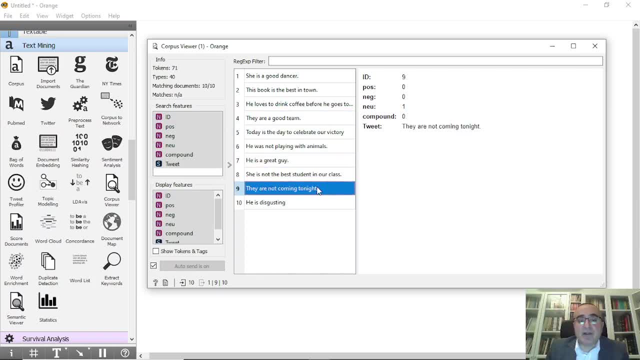 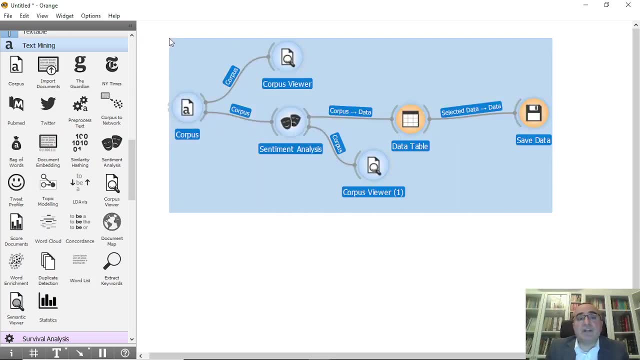 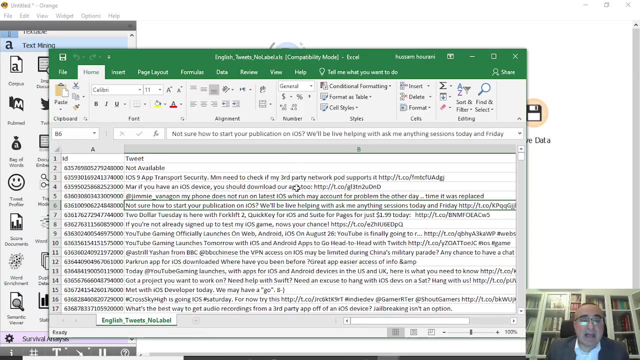 neutral and compound: see pair, each pair, each one. okay, so this is how you see the statements in sentiment analysis. so this is the first part I would like I wanted to show you. now let's also talk about the second part. the second part I wanted to show you is the tweets. we have tweets here and from the tweets, real tweets. 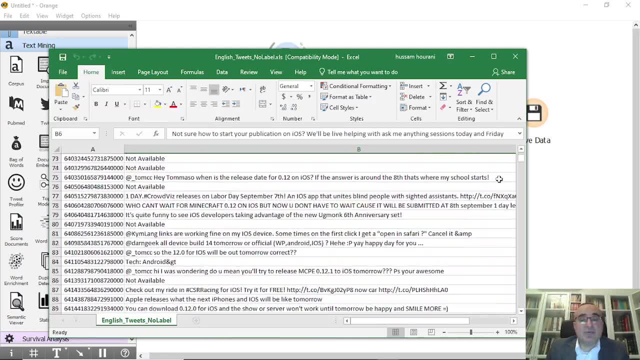 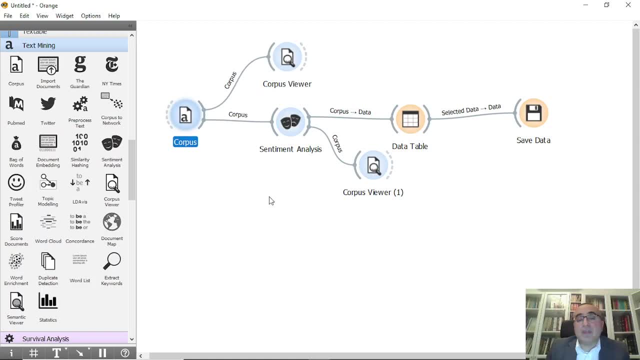 from Twitter. we would like to see the sentiment for all these tweets. this is a big file, okay, so let's try to play with this file and see how we gonna show the sentiment analysis. so I'm gonna click on corpus, corpus and from corpus, I'm gonna go and select the, the file I wanted to show you. 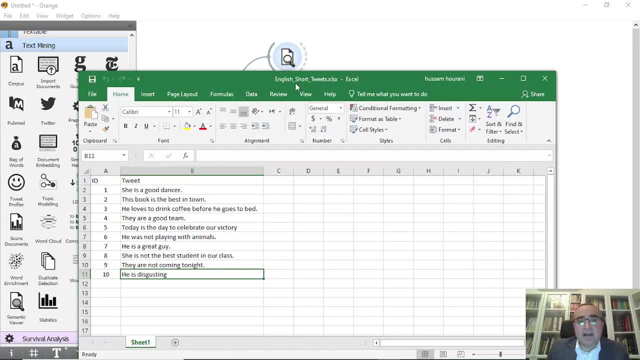 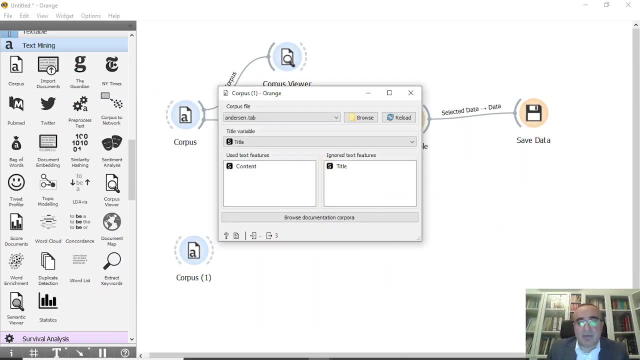 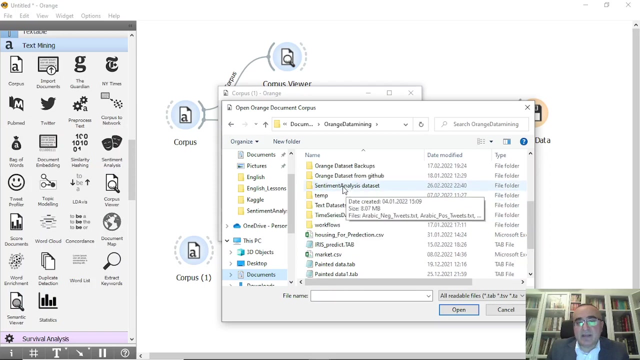 which is this file here naming English short tweets? not this one. but I need to choose the second second file, which is: which is this file? English tweets, no label. English tweets, no label. so I'm gonna go and browse this file. so I'm gonna go to sentiment analysis and from sentiment analysis, English tweets, no label. so we 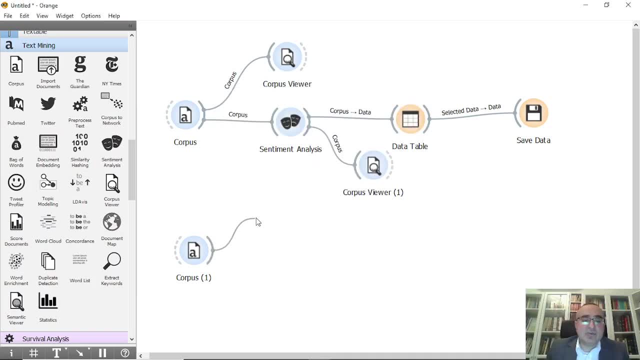 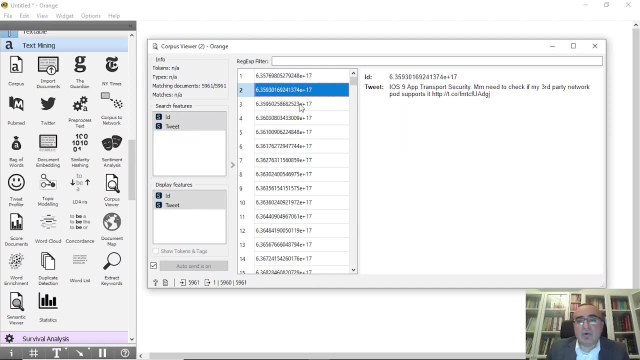 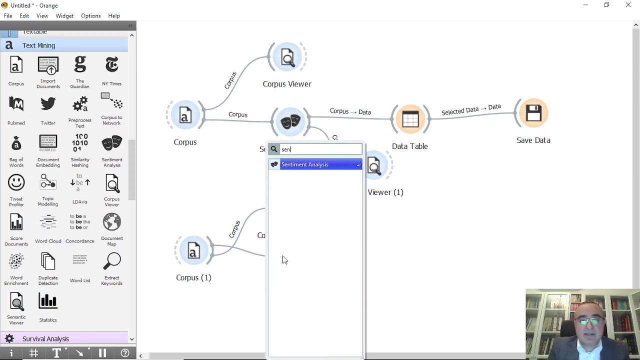 don't have labels for this one. so, uh, this is done. so now you can go to corpus viewer and from corpus viewer you can see all these. you know these tweets? okay, we have many tweets. we have five thousand six hundred, uh, five thousand nine hundred sixty one tweets, so now you can connect direct to sentiment. sentiment analysis. 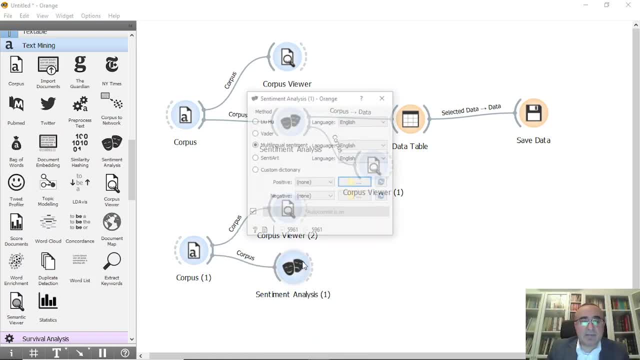 okay, and from sentiment, you can do the setup for you. you can choose the language, the multi sentiment method, you can use the Leo HU method and then you can choose the language. we have many languages here. see all these languages you can use. okay, and you can go into this one also. 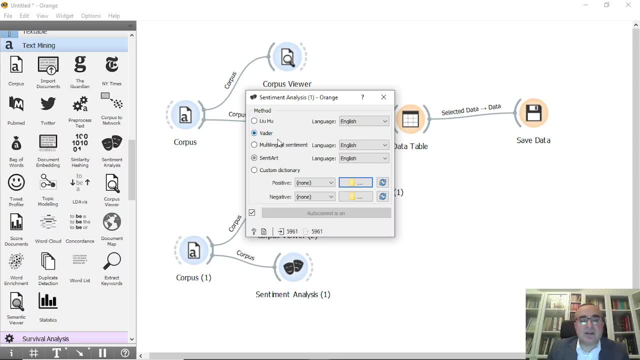 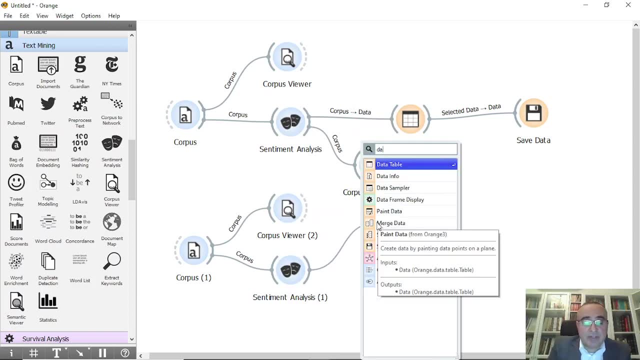 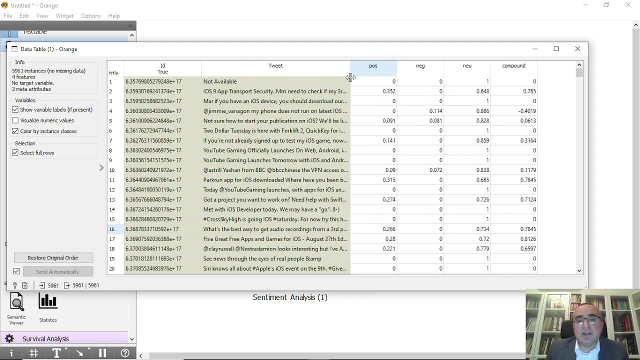 there is also different languages. let me use this one, for instance, because it's in English and it's straightforward with this one, so you can click, or you can go into data table okay and see all the tweets. these are the tweets, okay, IDs, tweets, and you can see the negative and positive. let's for example: 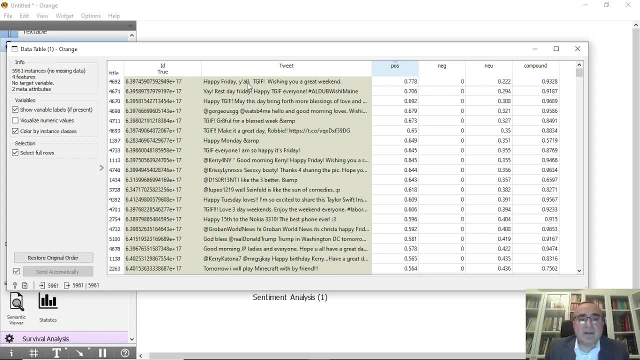 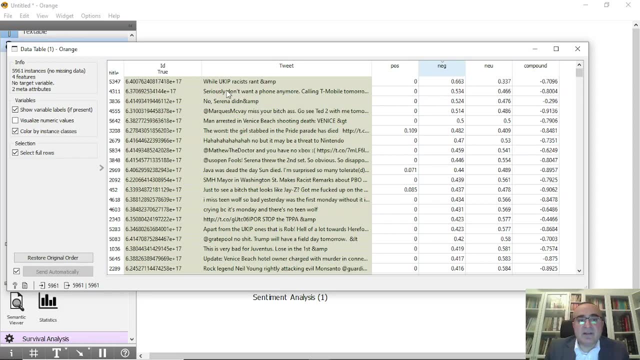 see the most positive words, which is this one: happy Friday you all, Etc, Etc. uh, you can also see the most negative words statements. uh, this is the definitely a negative statement. this is also a negative statement. also, this is a negative. all these are negative statements. okay, and this is the compound. 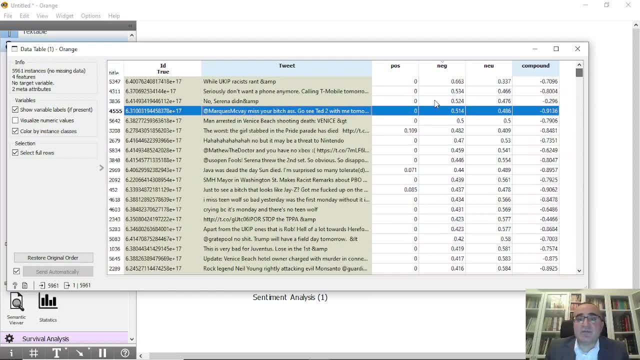 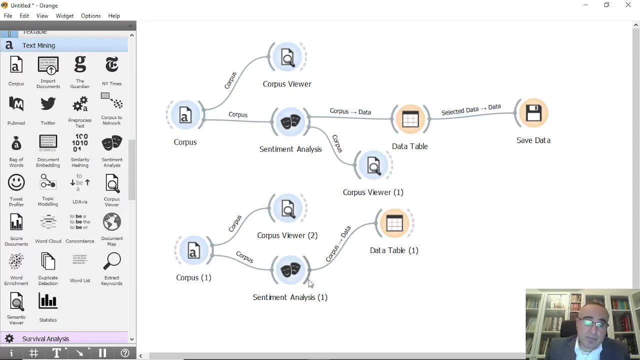 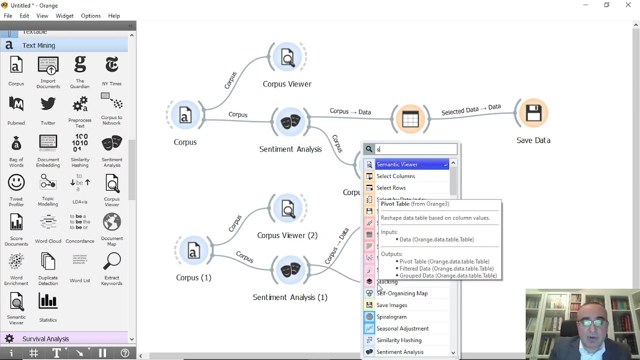 compound uh measures for all these statements. so, as you can see the positive, negative, neutral and compound. this is the first thing. also, I would like to see, uh, the heat map for this one. so I'm gonna, for instance, go and select columns, select columns, and from select columns, I will. 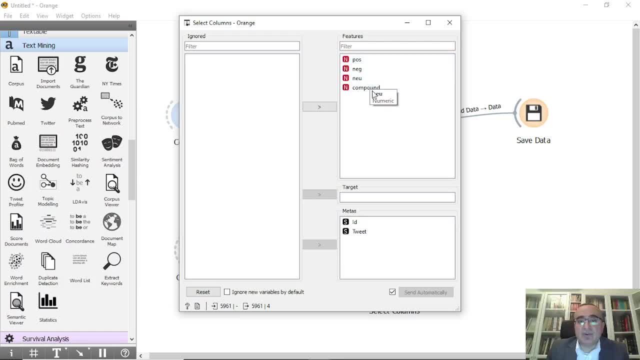 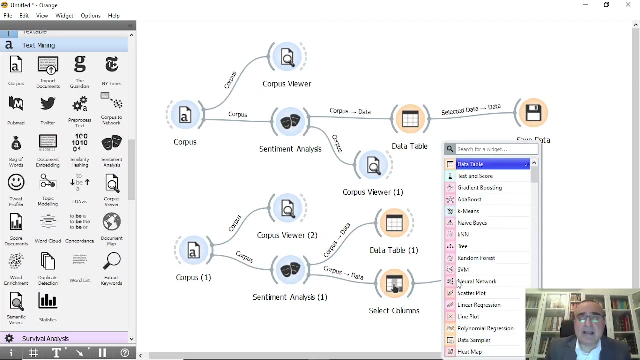 just use, uh, the positive, negative, neutral and compound, and I'm gonna move the ID tweets into meters, as you can see. I just want to see these in heat map, these four measures, okay, and from this you can also do sampling: sample sampler, data sampler. I don't want to see all the data. 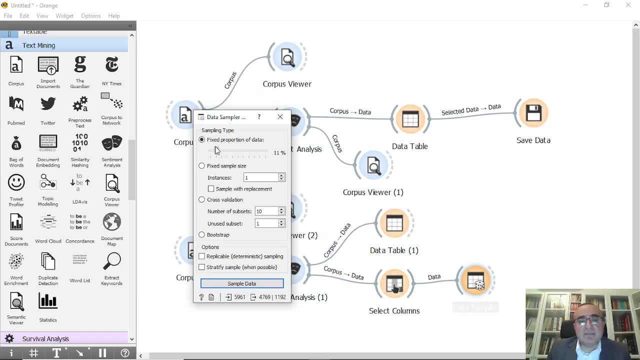 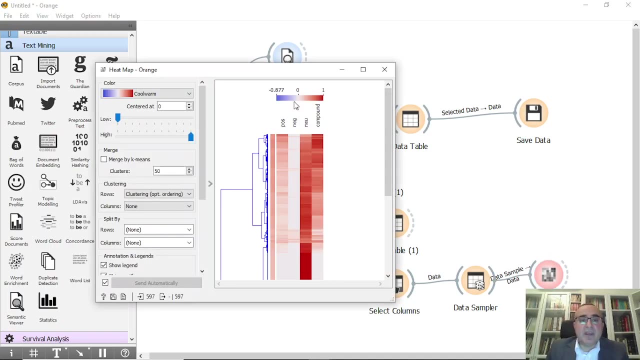 I want to use, for example, uh, 10 percent, this is the 10 percent, so this is it, and from here you can go to heat. heat map, okay, and from heat map: okay, it will take. yes, done so. from heat map, you can use the coloring schema, so the blue is negative and the red is positive. okay, as you can see you. 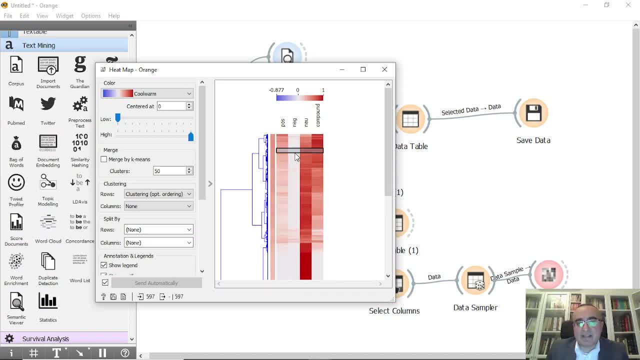 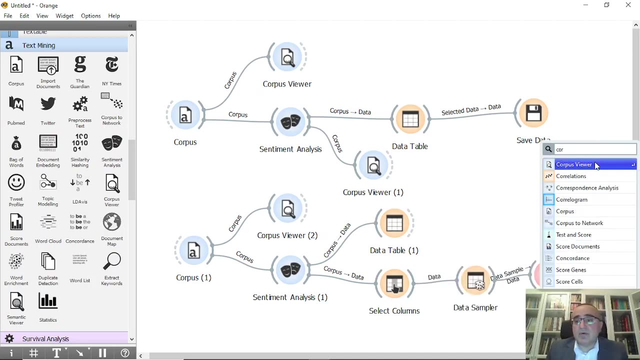 can choose whatever you want to see from here. for example, I want to see this part, or, for example, this and uh, or this part, smaller part, this part, for example. and from here you can choose the corpus viewer- okay, corpus viewer, and you can see all the documents and the tweets that relates to the to. 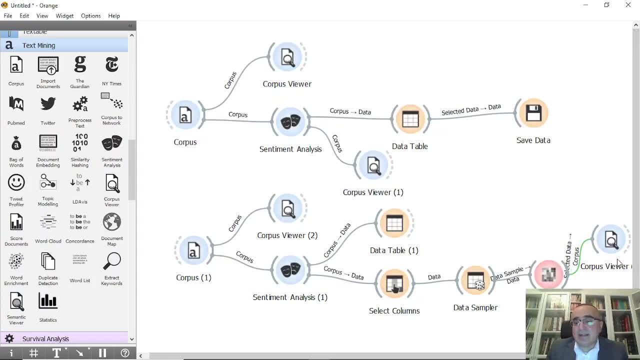 that part. okay to that part. and, as you can see, it's very straightforward. we've done sentiment analysis and, by the way, you can do some pre-processed pre-text before the sentiment, if you want. you can, for example, remove certain words, Etc, Etc. before. 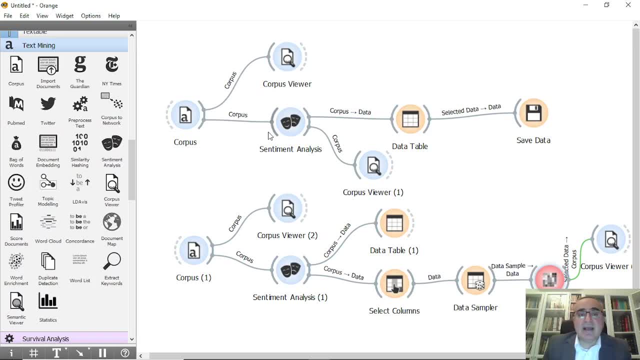 you do sentiment analysis directly, but this is a direct connection between corpus and sentiment analysis. but also you can do the pre-text format for the first example. you can, as I said, you can choose multi-sentiment analysis. this is English, so you can see the the results here. okay, the multi.